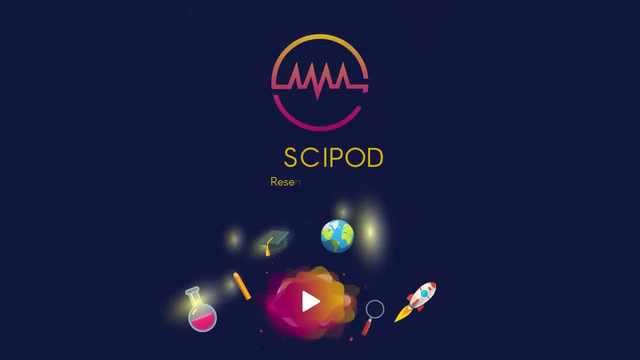 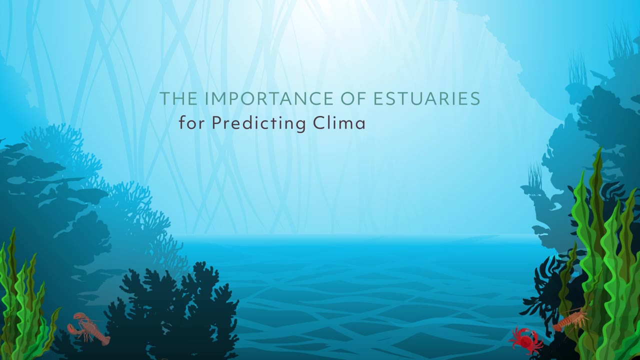 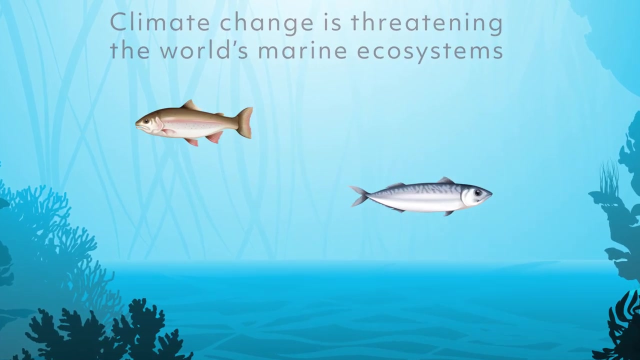 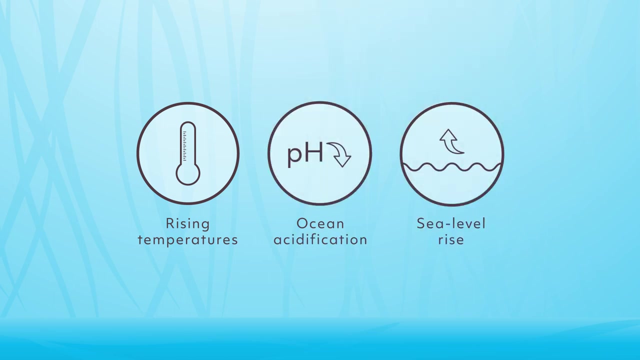 The importance of estuaries for predicting climate change impacts in the oceans. Climate change is threatening the world's marine ecosystems in myriad ways due to rising temperatures, ocean acidification and sea level rise. Another often overlooked effect is that warmer temperatures and changing weather patterns can alter the transmission of many 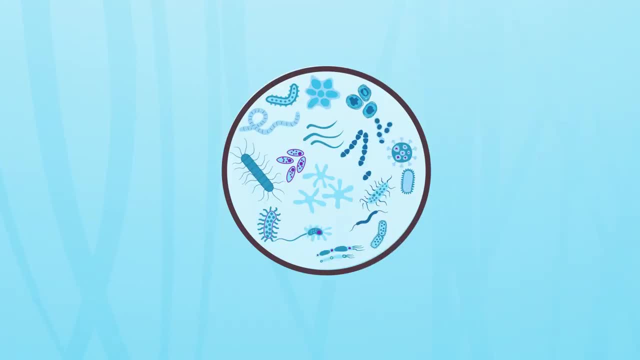 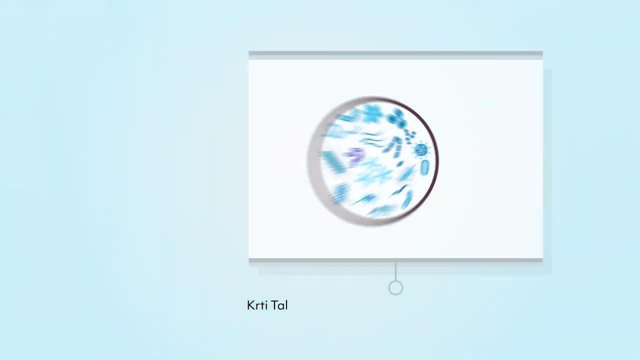 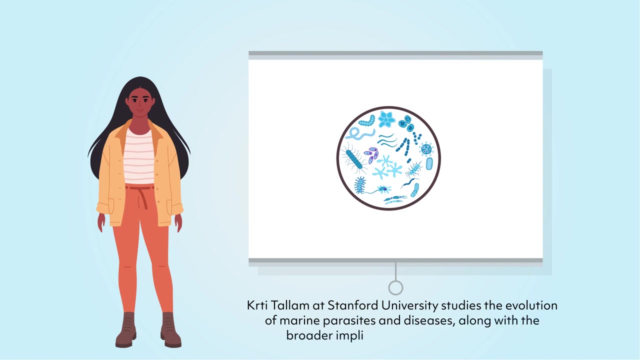 marine parasites and infectious diseases. Such diseases don't just impact their host populations, as cascading effects can disrupt entire ocean food webs. Kwethi Thallam at Stanford University studies the evolution of marine parasites and diseases, along with the broader implications for marine ecology. In a recent review paper, Thallam focuses on critically important ecosystems. 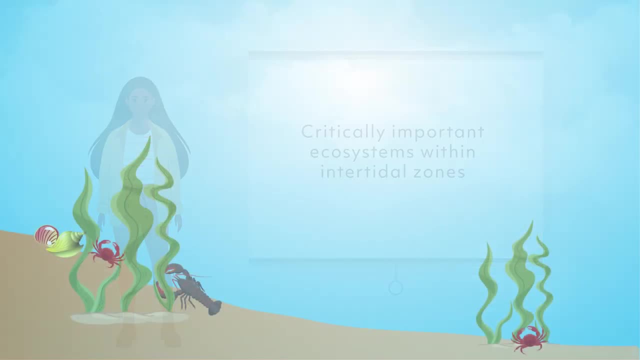 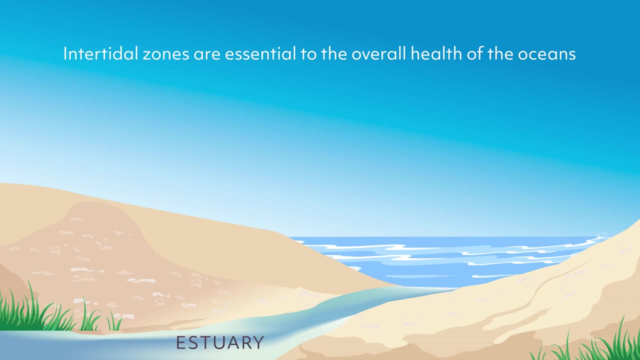 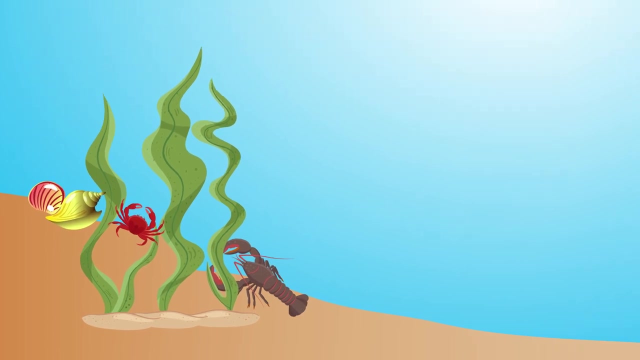 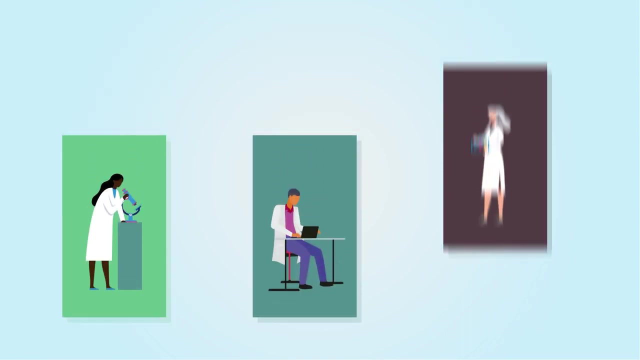 within intertidal zones. Estuarine species are useful indicators for monitoring climate change and diseases in both aquatic and terrestrial habitats. However, researchers who measure changes in estuaries often use different methods and work in diverse regions. These discrepancies make it difficult. 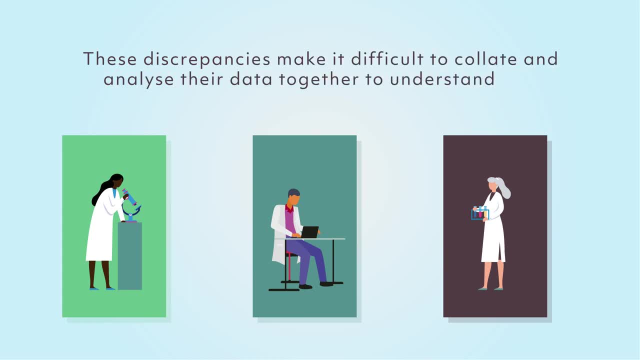 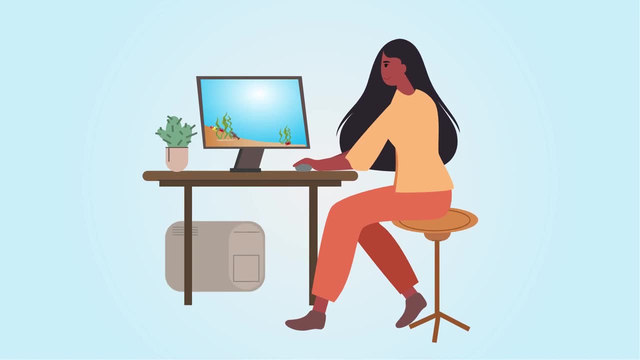 to collate and analyze their data together to understand how estuaries change over time, Towards creating a more standardized approach for tracking changes in estuarine ecosystems. Thallam investigated numerous studies published over the past two decades that measured intertidal health. 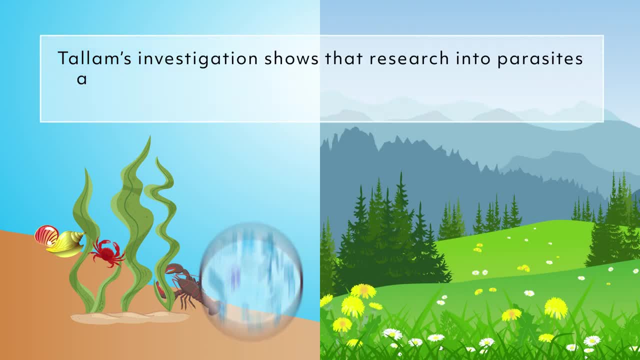 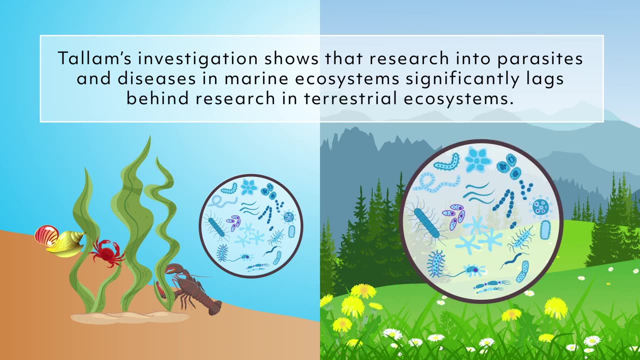 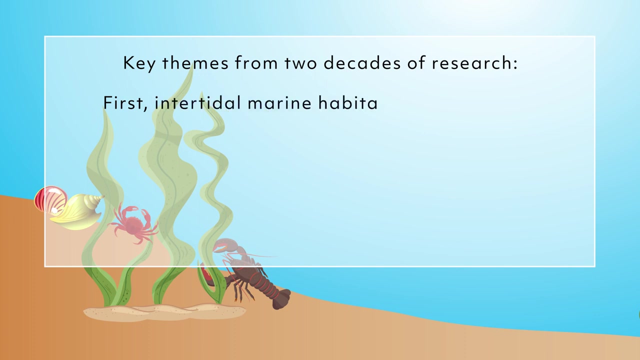 Thallam's investigation shows that research into parasites and diseases in marine ecosystems significantly lags behind research in terrestrial ecosystems. Despite this shortcoming, she was still able to reveal some key themes from two decades of research. First, intertidal marine habitats are likely to be most vulnerable to temperature increases.